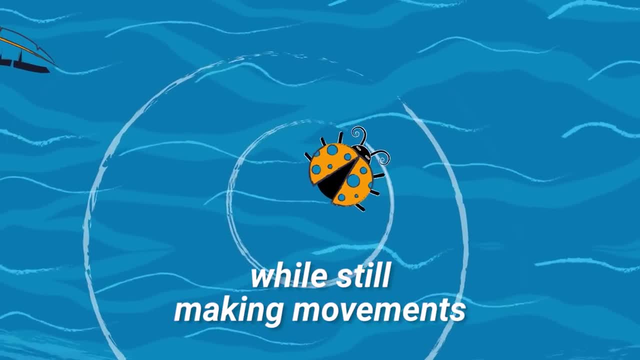 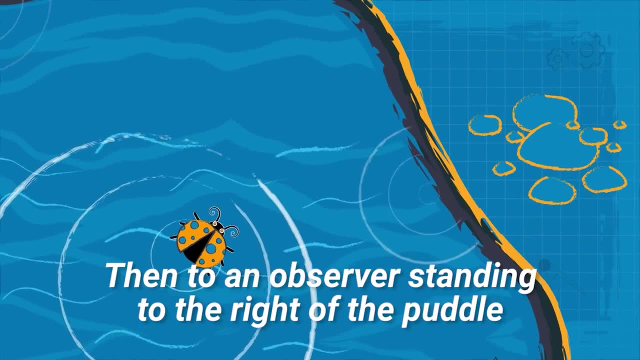 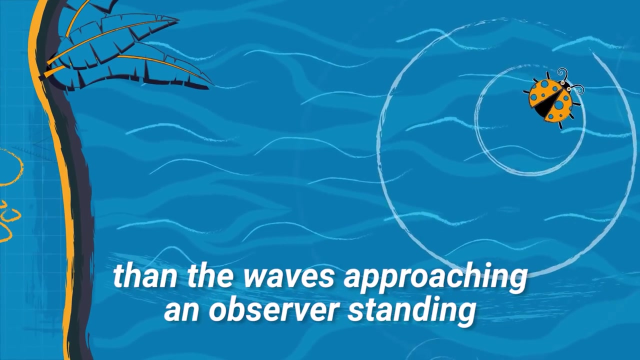 But what if the bug were to start moving toward the right, while still making movements with its arms and legs at the same frequency of once every second? Then, to an observer standing to the right of the puddle, the incoming waves would appear to be at a faster frequency than the waves approaching an observer standing to the left. 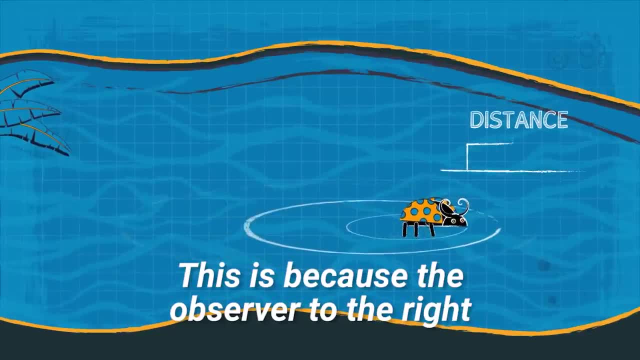 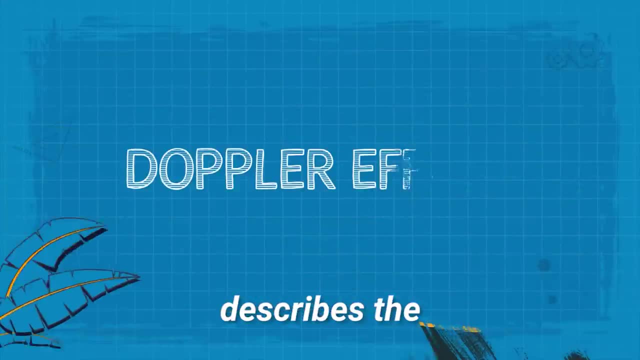 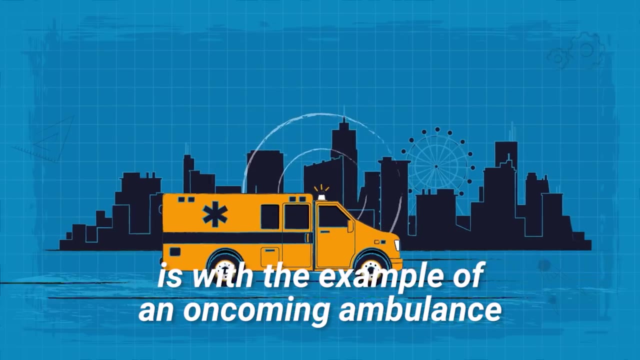 of the puddle. This is because the observer to the right is closer to the bug and therefore the waves. This in essence describes the Doppler effect. Another way to explain it is with the example of an oncoming ambulance. When an ambulance approaches you, its siren has a higher pitch as it is approaching than 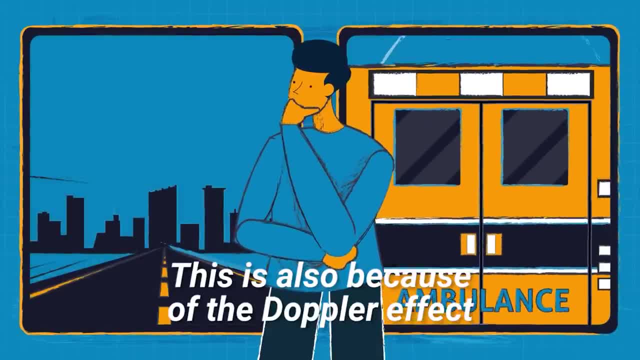 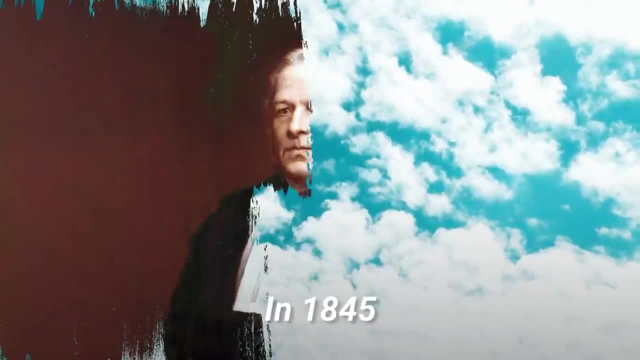 when it is moving away. This is also because of the Doppler effect. It might seem simple and self-evident, but it is an important concept. In 1845, Dutch chemist and meteorologist Dr J S Schubert came up with the idea. 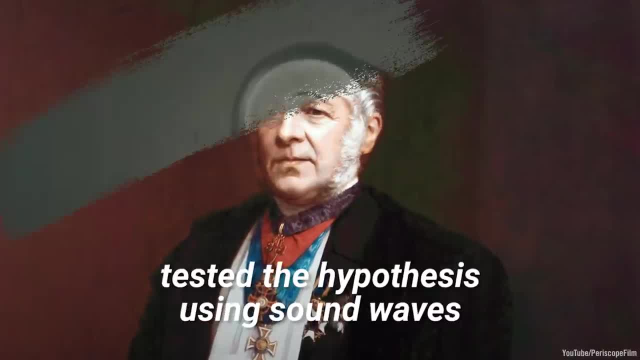 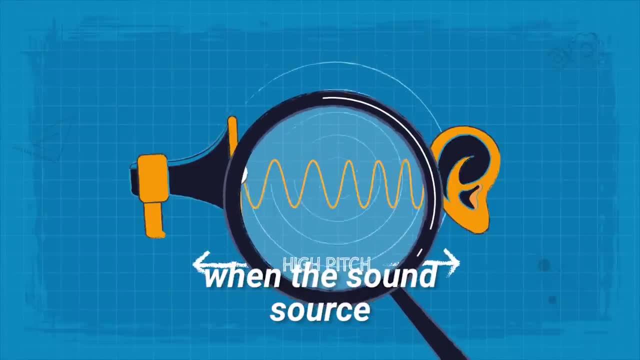 of the Doppler effect. The Doppler effect is an important concept. A scientist, Bayes Ballot, tested the hypothesis using sound waves. He found that a sound's pitch was higher than the emitted frequency when the sound source approached an observer and lower than the emitted frequency when the sound 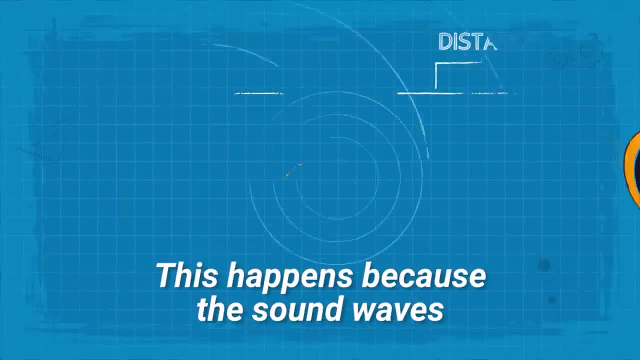 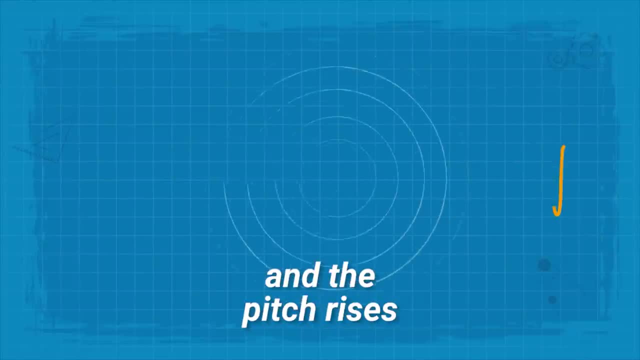 source moved further away from the observer. This happens because the sound waves compress as they approach the observer. This increases the frequency of the wave and the pitch rises. As the waves recede, the observer will hear a lower pitched noise. This can increase the frequency of the wave and the pitch rises. 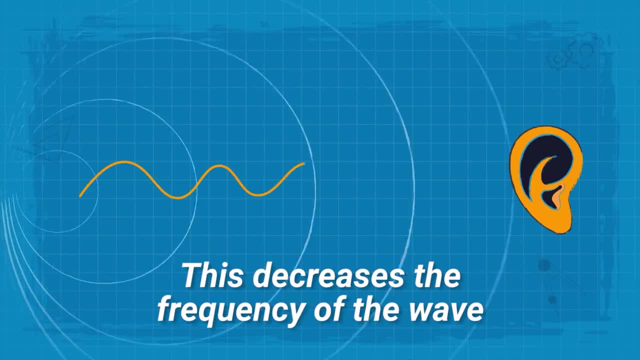 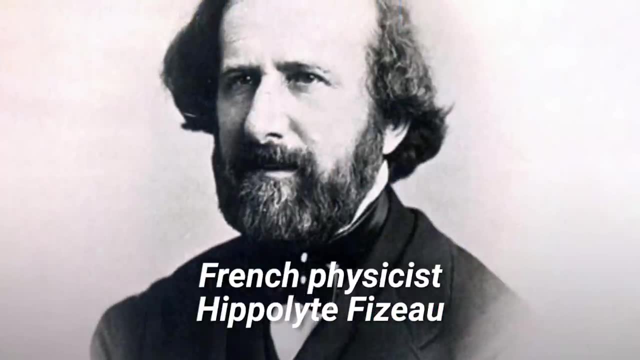 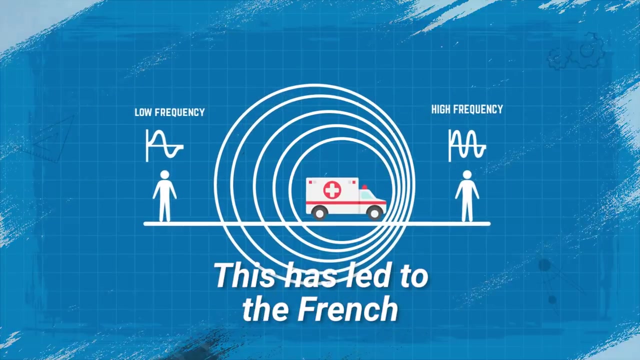 pitch noise because the sound waves stretch out. This decreases the frequency of the wave and the pitch falls. Meanwhile, French physicist Hippolyte Fizeau also stumbled independently on the same phenomenon in 1848.. This has led to the French referring to the Doppler effect as the Ife-Doppler Fizeau. 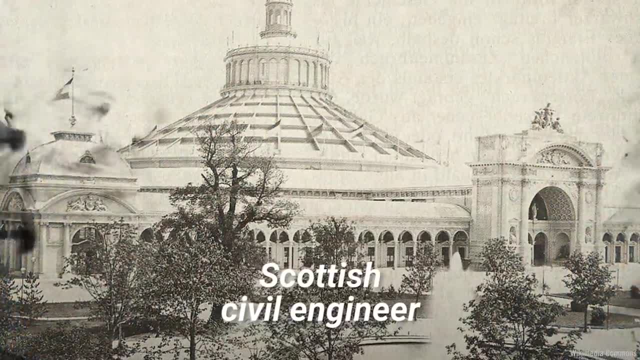 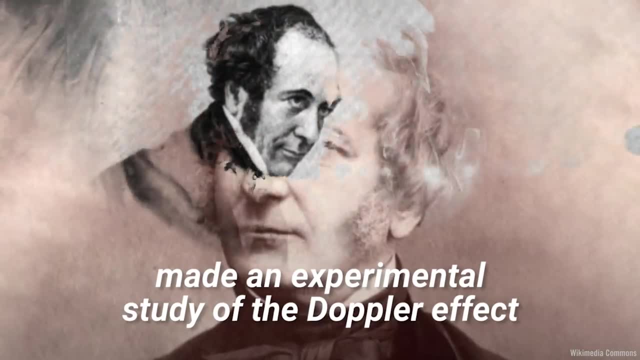 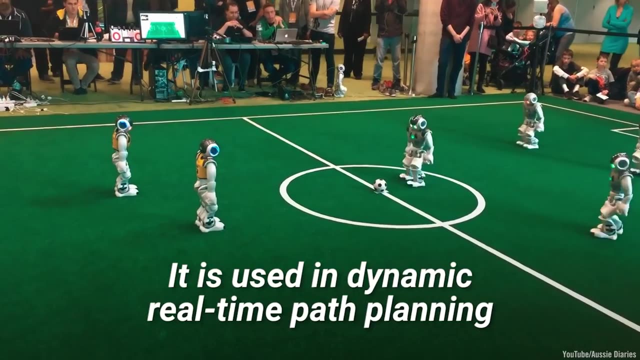 Finally, also in 1848, Scottish civil engineer, naval architect and shipbuilder, John Scott Russell, made an experimental study of the Doppler effect that proved Doppler's theory. Today, the Doppler effect even has applications in robotics. It is used in dynamic real-time path planning to help in the movement of robots, such as: